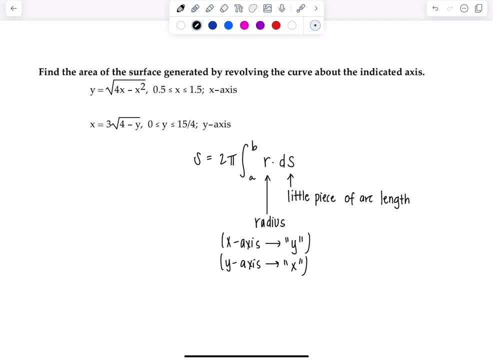 lecture video. I'll put the link in the description. But basically you can integrate with respect to either x or y. It just really depends on what sort of equations you're given. Okay, so, like for this first example right here: Okay, y equals square root of 4x minus x squared. So already y is given. 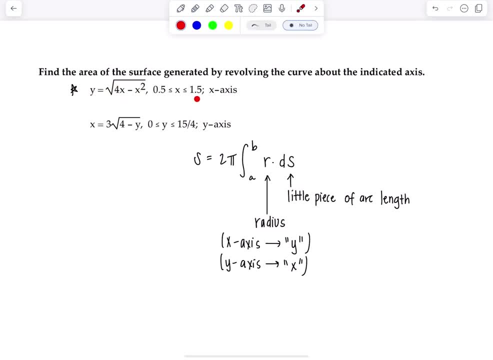 as a function of x. The limits are in terms of x. So let me see if I can just integrate with respect to x and leave everything as is. Since I'm spinning around the x-axis, the radius is going to be y. I can't leave y in my integral. You're not in multivariable calculus yet. So if everything, 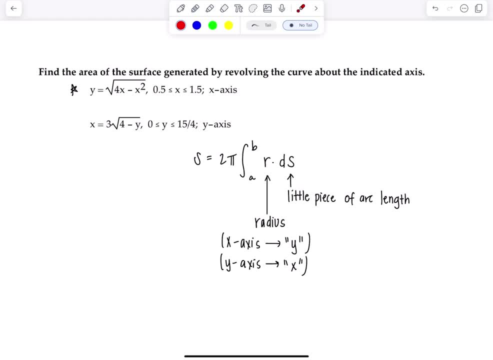 else is in terms of x, then r, which is y, You're going to replace with the function given. Okay, let us set it up. So again, let me iterate, reiterate: ds has two options. Its arc length, it can be square root of 1 plus dy, dx, squared dx or 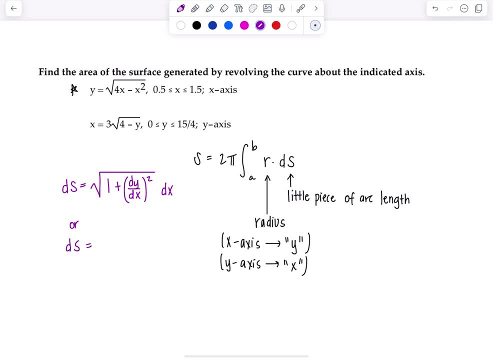 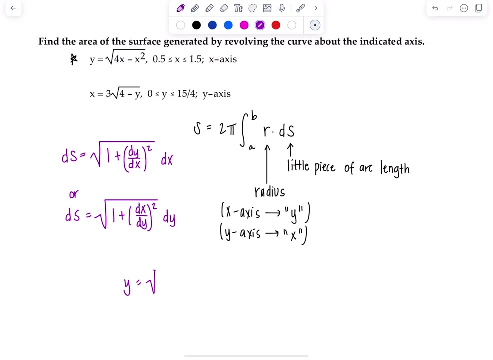 it can be square root of 1 plus dx, dy, squared dy, Depending on what you're doing. Okay, so this first one here we have, y equals square root of 4x minus x. squared x is from 0.5 to 1.5 and we're spinning about the x-axis. So that tells me right away the radius is y. 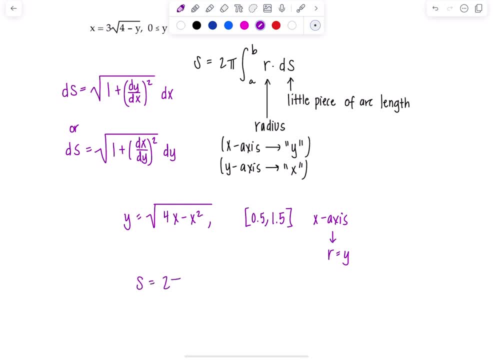 So let's set it up: Surface area equals 2 pi. Limits are from 0.5 to 1.5.. The radius is y, and then we're spinning about the x-axis. So that tells me right away: the radius is y. 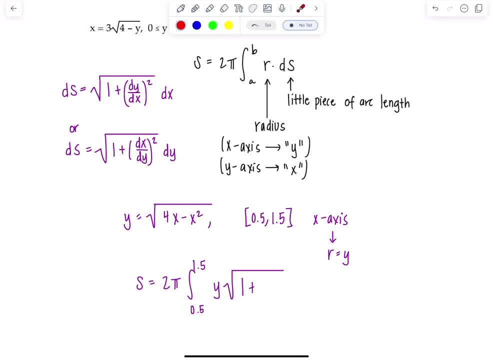 We have square root of 1 plus. Since everything is already set up, y is a function of x, I'm just going to leave it and write this as dy, dx, squared dx, And then that tells me: okay, if I'm integrating with respect to x, these limits better be in terms of x, which they are, And then y. I can't leave it. 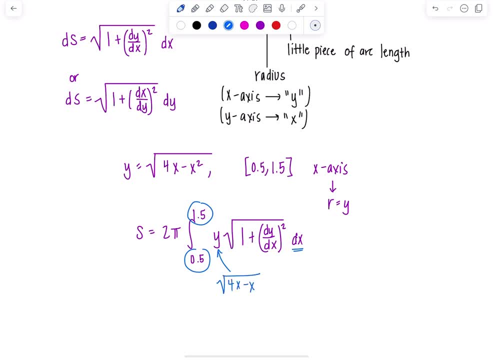 like that. I'm going to have to replace it with 4x rad, 4x minus x squared. You see, Okay, I like to do all my prep work before I set up the integral. So I like to compute 1 plus dy dx squared. 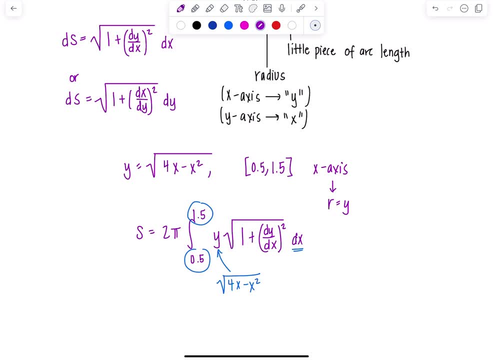 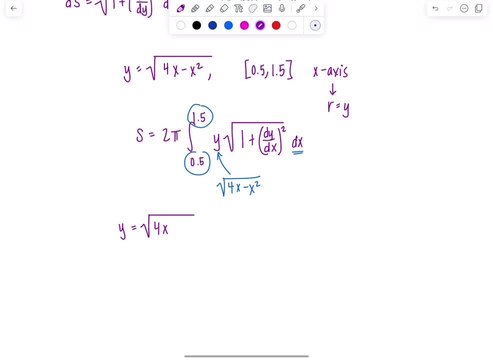 Clean it up as much as possible and then start writing out the integral. So y is rad 4x minus x squared. Let's go ahead and take the derivative. So dy, dx. And I teach my class this useful little shortcut: If you have the derivative of a square root function, that's a composition, you put 2 and 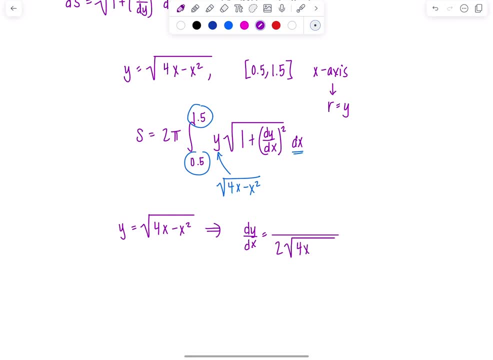 the original radical in the denominator, And then you put 2 and the original radical in the denominator, 4x minus x squared, And then we have to use the chain rule, right? So I need to multiply by the derivative of what's underneath the square root sign in the numerator, And that's just going to. 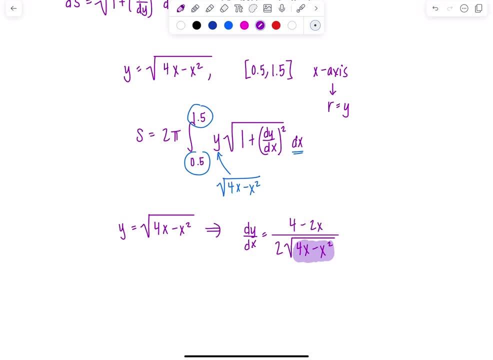 be 4 minus 2x, And then I can clean this up, because if I factor out a 2 here, then I have 2 minus x, And this 2 cancels with the 2 in the denominator. So now we have 2 minus x. 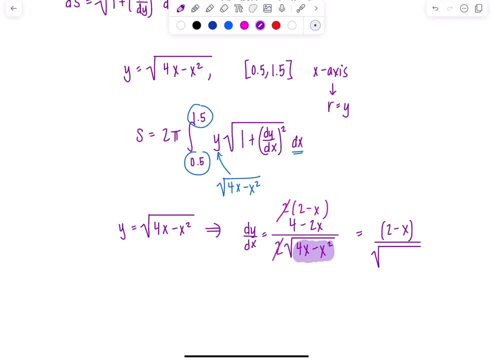 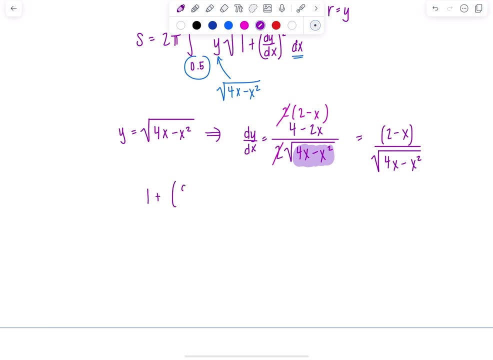 squared over square root: 4x minus x squared. Okay, so then that means 1 plus dy. dx squared would just be 1 plus. I'll write this as 2 minus x squared over. Now we have no more radical, It's just going. 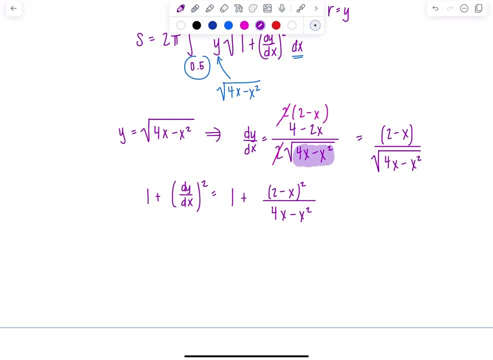 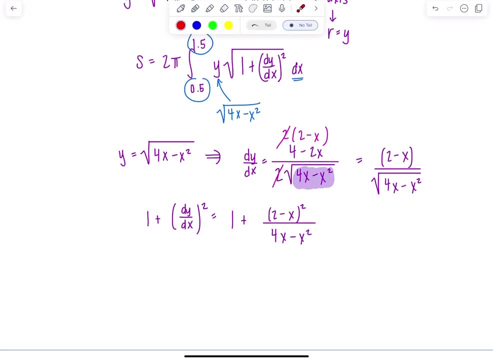 to be 4x minus x squared in the denominator, And I usually just stop right there. Yeah, I sure do. So let's look back at our integral setup here with the formula. I think we're ready. I'm going to replace 1 plus dy, dx squared with all of this loveliness, And then replace y with the function. 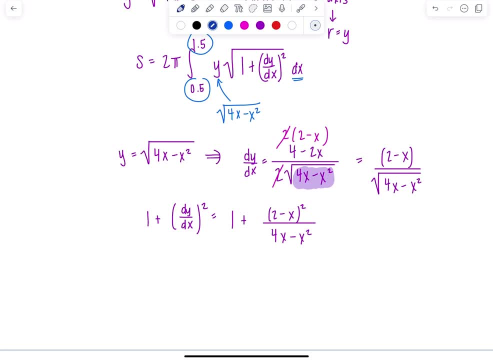 that we were given. Okay, are you ready? Here we go. So surface area- Excuse me, It's very early in the morning. 2 pi times the integral from 0.5 to 1.5.. Y we're going to replace with radical 4x minus. 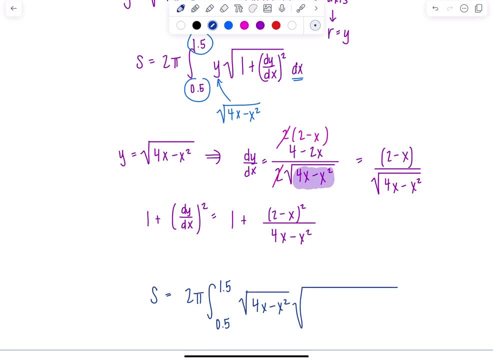 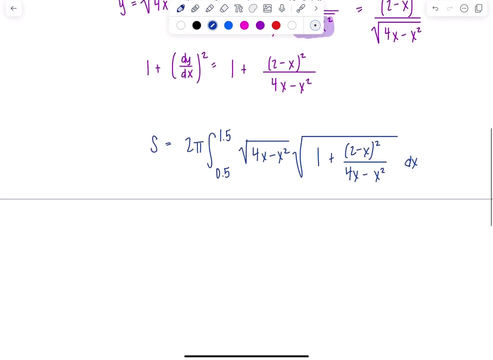 x squared. And then I have another big radical of 1 plus 2 minus x, squared over 4x minus x, squared dx, like that. Okay. now the next step is like a common little trick that you have to do with these surface area problems. Okay, you actually combine both of these radicals under one big one and 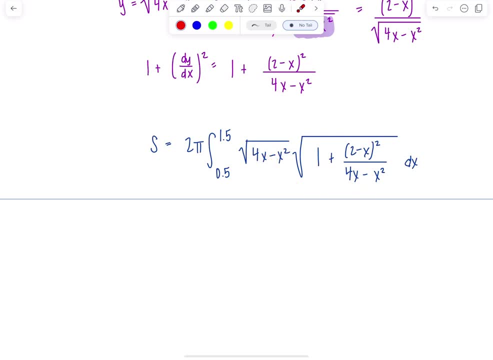 you're going to distribute This radical through to the other stuff, So watch, I'll do it step by step, in case this is your first time seeing such a thing occur. Big radical. Then you have 4x minus x squared times what was already. 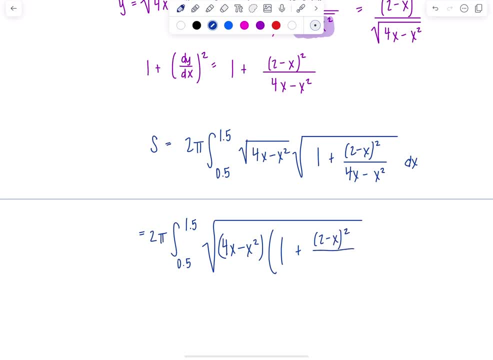 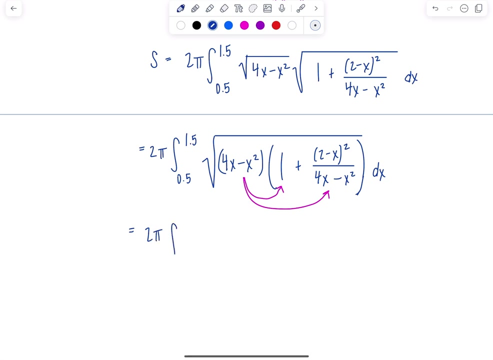 there: 1 plus 2 minus x, squared over, 4x minus x squared Close it. Don't forget the dx. Okay, Now, here's where it gets so lovely, because I'm going to distribute, distribute, And perhaps you can already tell some lovely cancellation will occur. Right, 2 pi integral 0.5 to 1.5. 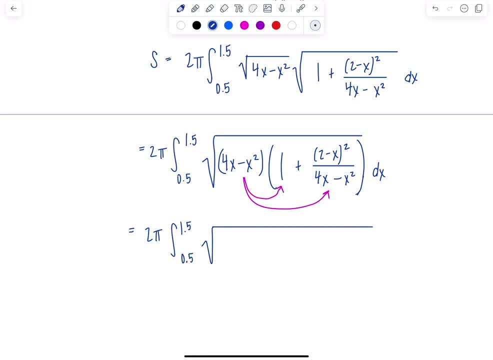 square root. 4x minus x squared times 1 is just itself Plus. and then now when I distribute 4x minus x squared to the second term, I get the integral. So I'm going to distribute this in those prime brackets over 5 and then I'm going to distribute this in theкими Plus times 5 times. 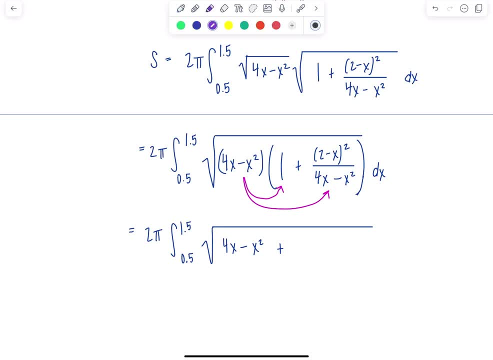 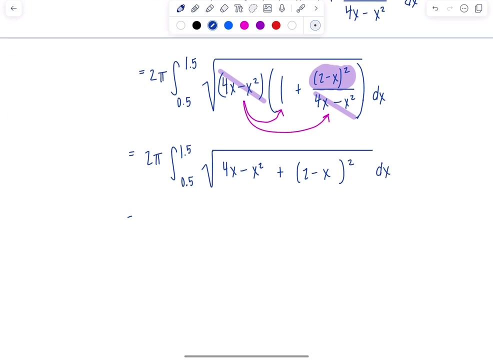 the was deles times. plus are plus. Now that's going to be where parked right now, Just kind of the second term. Look what happens. It's great. It cancels with the denominator and I'm just left with the quantity 2 minus x squared dx. Okay, now, underneath the radical, you just have a little foil. 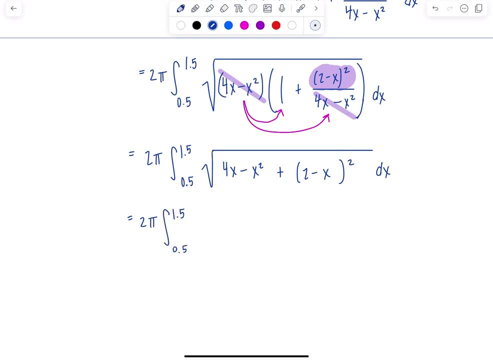 party 2 pi 0.5 to 1.5 square root. what's this? 4x minus x squared plus 4 minus 4x plus x squared dx. Oh, look at this more canceling fun. 4x is gone, x squared is gone. We only have rad 4 left. 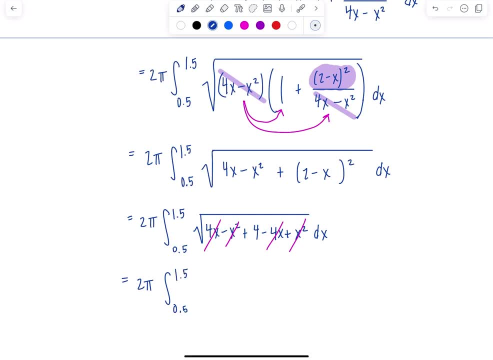 Yes, it's like once you get to this point, the integral is so nice. So did you? you observe? All I have left is square root of 4, which is 2 dx. Antiderivative of 2 would be 2x. 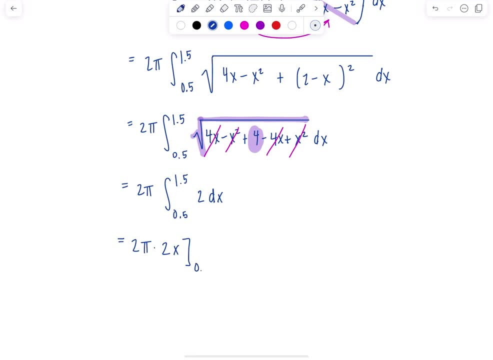 So I have 2 pi times 2x, evaluated from 0.5 to 1.5.. You can just group all these constants together, So it's 4 pi times evaluating x, upper limit minus lower limit. That's just 1.. 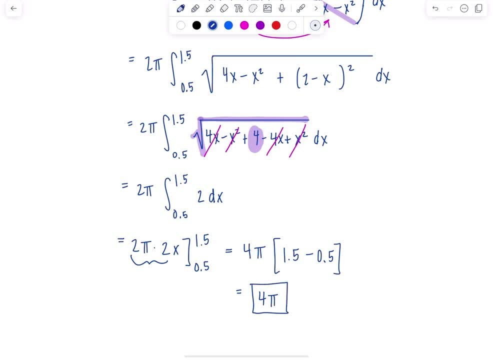 So this final answer is just 4 pi, And I always like to write that this is units squared, Just to remind myself this was surface area. So we're finding a two-dimensional answer. Okay, how was that? Did you love it? Now let's look at another one This time where we're going. 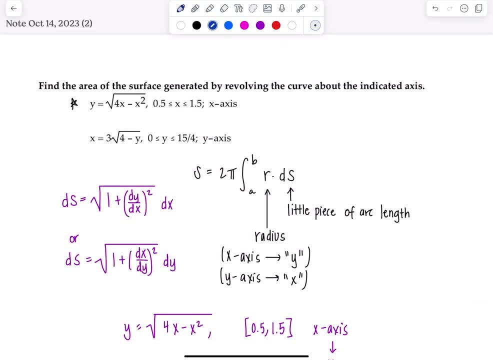 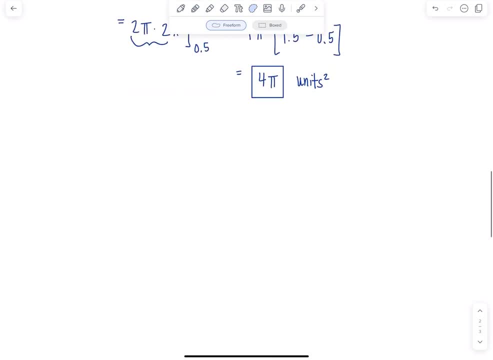 to have to set it up differently. So you have some options. Let me copy this down below. So again, surface area. You notice this is different because x is given as a function of y, Okay, and my limits are in terms of y. If we're spinning around the y-axis, that means my radius is x, So surface area is. 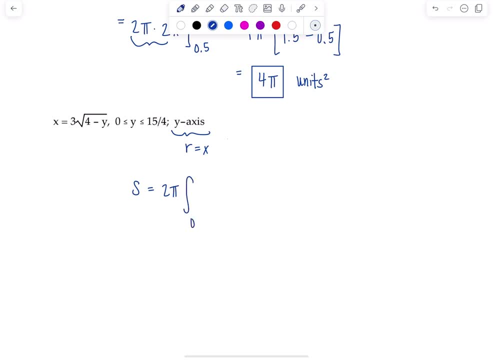 going to be 2 pi. I have 0 to 15 over 4, x times the square root of 1 plus dx dy squared. And notice, I'm in good shape. If I'm going to integrate with respect to y, I have to differentiate with respect to y and the limits are with respect to y. 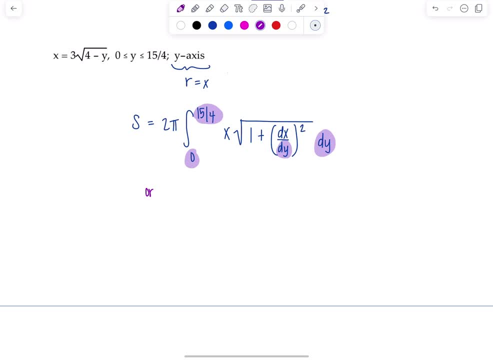 Now, if you wanted, if you wanted, when I gave this problem in class the other day, some students set it up differently. The radius still has to be x, That does not change, But they wanted to rearrange this equation and actually still find dy dx. 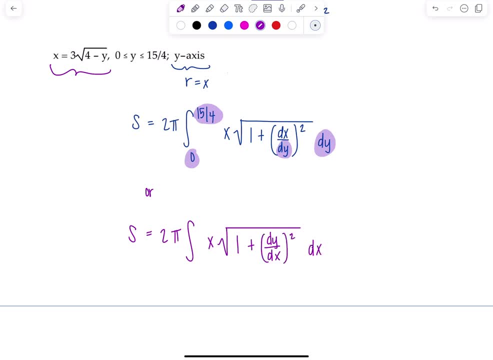 And integrate with respect to x, And that's totally fine. But the only issue is then that your limits also must match and be in terms of x, So you can find them. If y is 0, just plug it in here. So x of 0 is 3 rad 4 minus 0. So 3 times rad 4 is 3 times 2. So 6.. This would be a 6.. 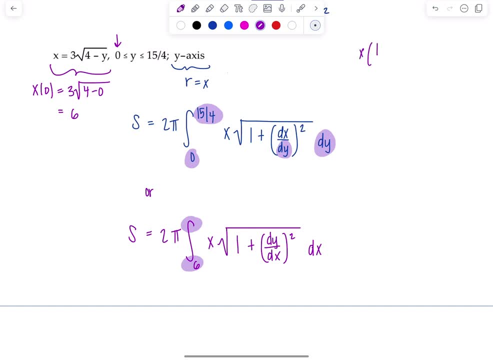 And then x of this is probably not going to be fun- x of 15 over 4. So it's 3 times square root. I'm already thinking this is 16 over 4 minus 15 over 4.. That's 3 times rad 1 4th, So 3 halves. Oh, that wasn't so bad. So upper limit is 3 halves. 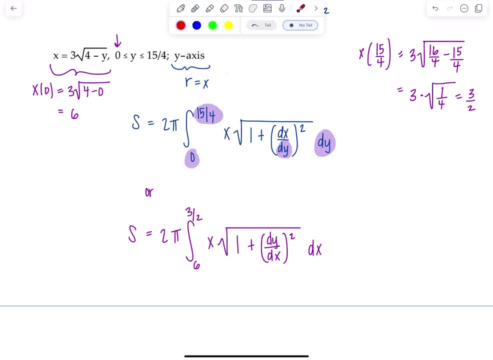 And then this is what I want you to observe now: Okay, If we go this route, I have to rearrange, get y by itself, take the derivative and you're good If we integrate using this option. here, in terms of y, I have to replace x, because everything must be in terms of y in the integral. 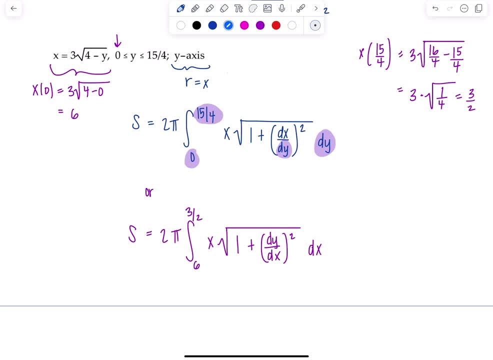 with 3 times rad, 4 minus y. It doesn't matter which one you do, They will come out the same And it will only differ, maybe at the end, when integrating, what technique you have to use. So just you know, in this case, if you want. 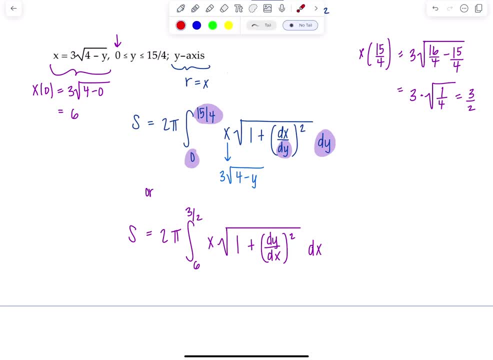 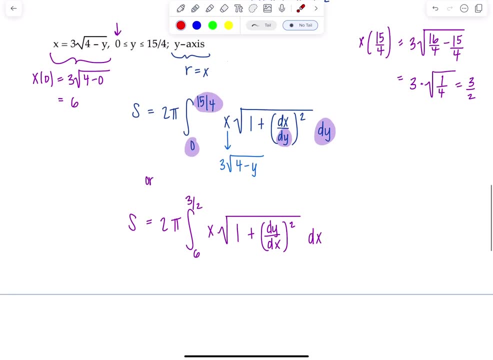 to try both ways. I'm going to just do the top one, because we already integrated with respect to x, Let's integrate with respect to y. But you can try this setup on your own. Okay, I had a few students do it. They were just 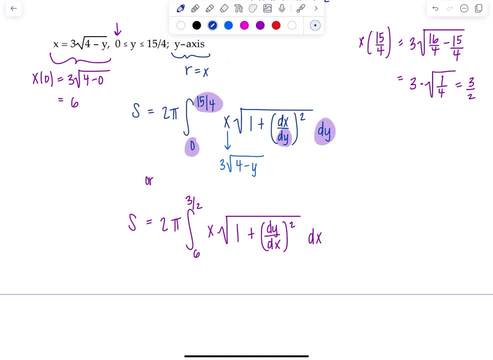 very moved to only integrate with respect to x, for whatever reason. So, x, what an ugly x Hold on. x equals 3.. I'm going to write this as 4 minus y to the 1 half. Yeah, So dx dy. 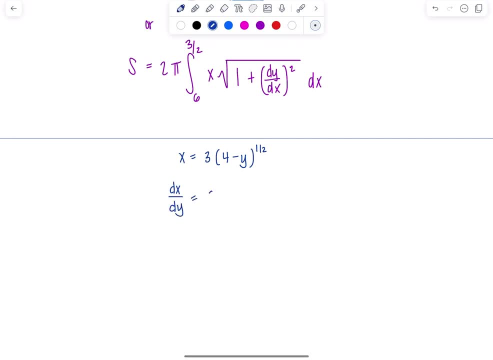 is going to be 3 times a half, So 3 halves, 4 minus y to the negative 1 half, And then by the chain rule. I'm going to write this as 4 minus y to the negative 1 half, And then by the chain rule. 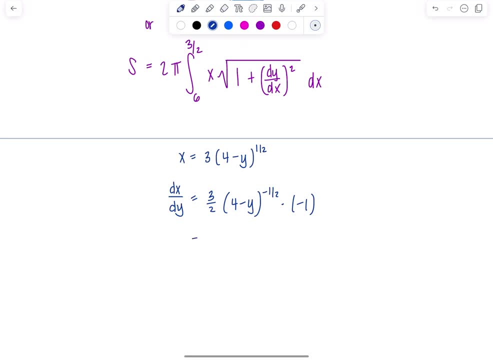 I have to multiply by the derivative of the inside, which is negative 1.. So this gives me negative 3 over 2 square root, 4 minus y. I didn't use the shortcut to take the derivative just now in case some of you hate it. And then that means 1 plus dx. dy squared would be 1 plus square the. 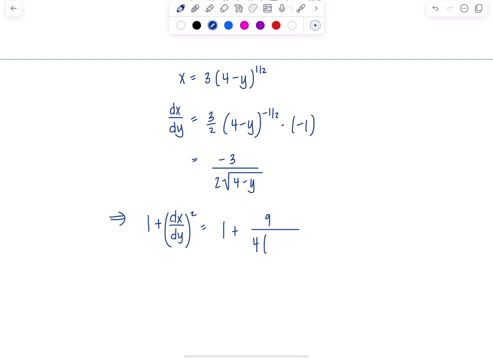 top: It's now 9.. Square the bottom: It's now 4 times. no more radical: 4 minus y. Leave it, Please leave it. I don't clean up much more from here. So surface area is going to be 2, pi Limits are from 0 to 15. 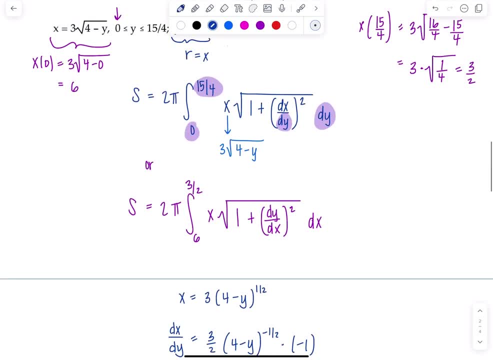 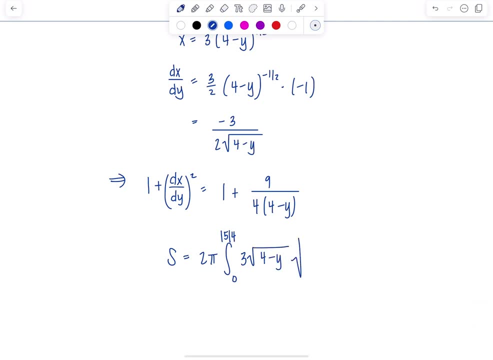 over 4.. Instead of writing x, I'm going to write 3 rad 4 minus y, 3 rad 4 minus y, And then we have big square root with everything from the line up above. And then, do you notice, we're at the. 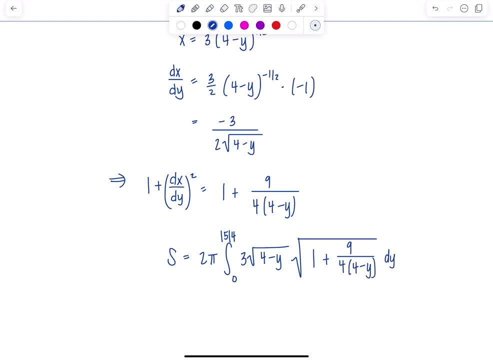 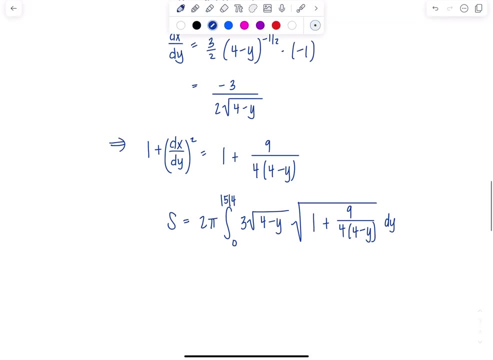 same point. We're going to use the same technique right now. So I'm going to come through, put this and this expression under the same radical and distribute the 4 minus y And, while I'm at it, take the 3 out with the 2 pi. Let them hang outside of the integral Become: 6 pi 0 to 15. 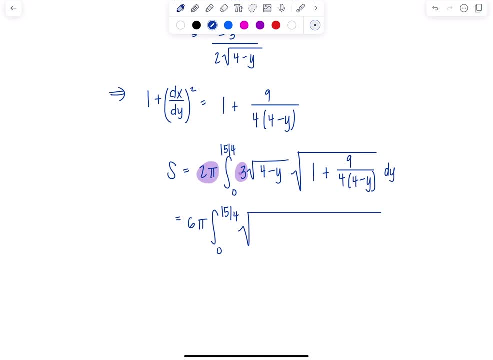 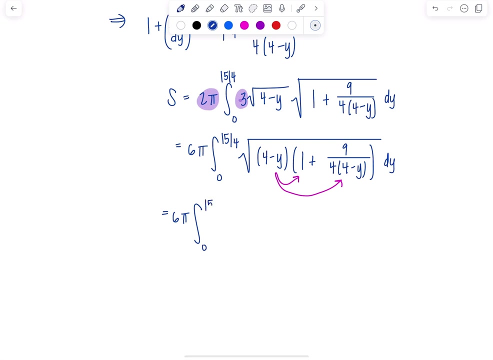 over 4.. Big radical. Here we go: 4 minus y times 1 plus 9 over 4 times 4 minus y, Et voila. And then this is the point where we distribute and it gets fabulous. So we have 6 pi integral 0 to 15. 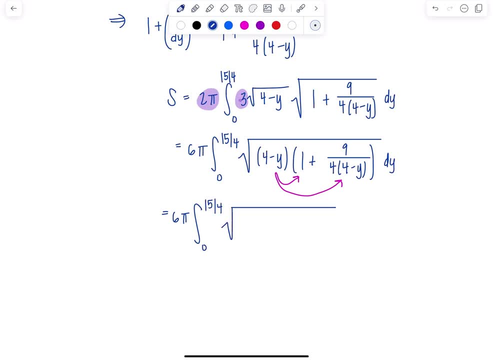 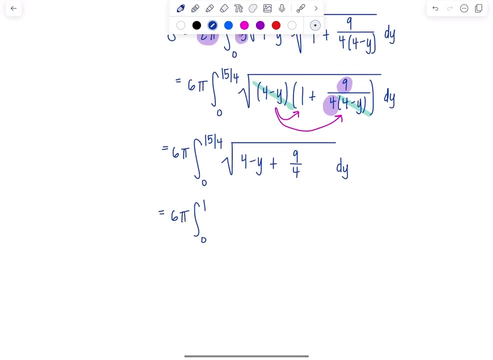 over 4.. Square root: 4 minus y plus. This 4 minus y cancels with the 4 minus y in the denominator, And then all I'm left with is 9 over 4.. And then dy. Okay, Cleaning up a wee bit more. This is 6 pi integral from 0 to 15 over 4.. 4 is 16 over 4 plus. 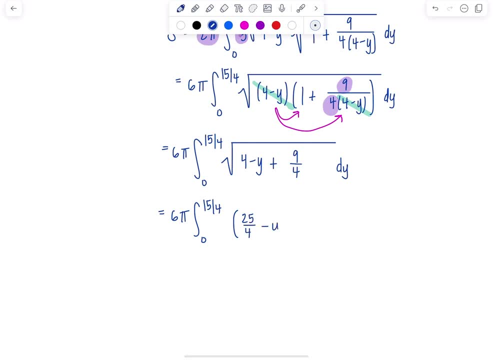 9. That's 25 over 4 minus y to the 1 half power dy. Now, if you need to to keep going, you could do a? u substitution. Let u equal 25 over 4 minus y. du would be negative 1 dy. So. 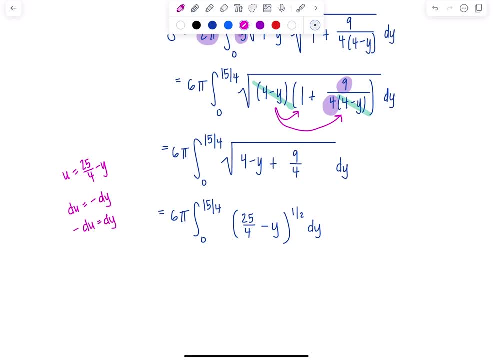 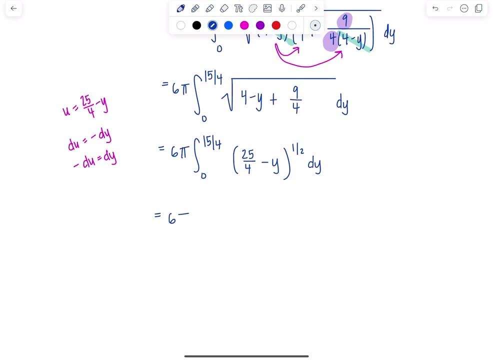 negative. du is dy Trying to get my students to think through that a little bit on their own and not actually have to do the? u substitution, Because then you got to change the limits and all that. Let's just see if we can leave it. It's going to be great. So 6 pi I know if I did the? u. 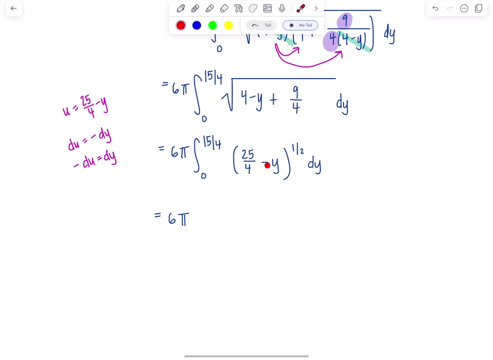 sub and everything. all that's going to happen is I'm going to pick up an extra negative, Basically because of the negative in front of the y, So I'm just going to, I'm going to put it outside the 6 pi. 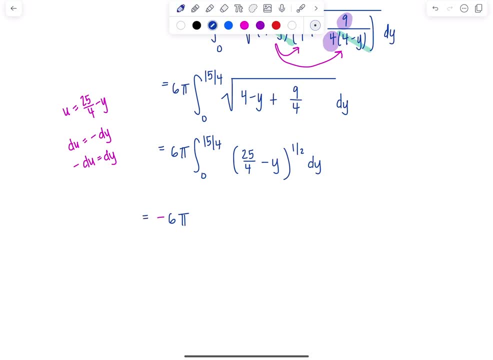 Right now like this: Okay Handled, Then currently this quantity is being raised to the 1 half power. So when we take an antiderivative we add 1 to the exponent, So it would be 3 halves And then. 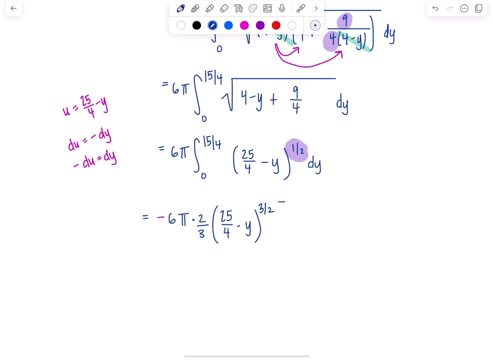 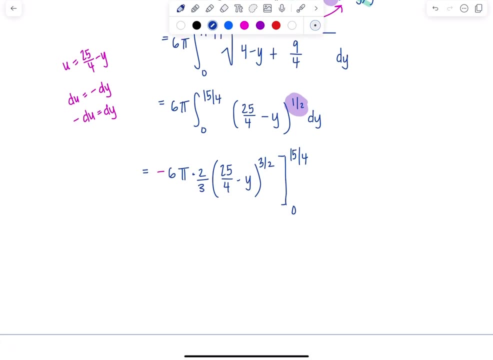 I multiply by the reciprocal of the new exponent And I'm going to evaluate all of this from 0 to 15 over 4.. Cool, This 3 cancels. Now this is a 2. Negative 2 pi times 2 is negative 4 pi, And then we have 25 over 4 minus. I'm going to plug in the upper limit: 15. 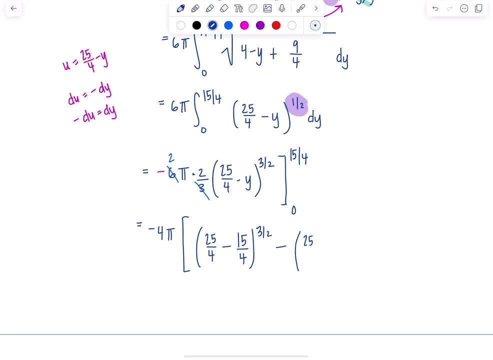 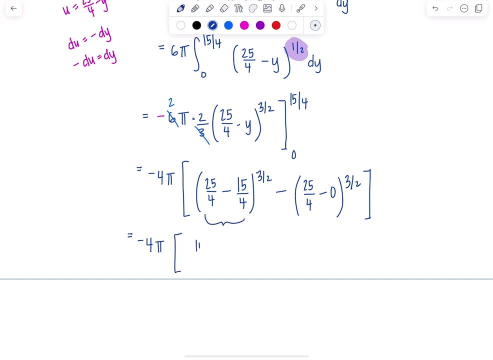 over 4 to the 3 halves, Minus 25 over 4, minus 0 to the 3 halves. That was ugly. There we go. So let's see This is negative 4 pi times. Here I'm going to have 10 over 4 to the 3. 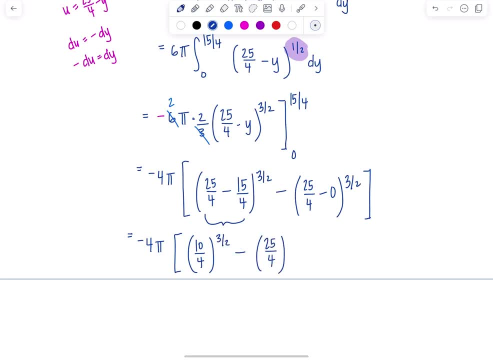 halves Minus 25 over 4 to the 3 halves. Now when you raise something to the 3 halves power, it means you take the square root and then you cube it. Okay, So this is negative. 4 pi times square root of 10 cubed would be 10. rad 10 over square root of 4 is 2, cubed makes it 8.. 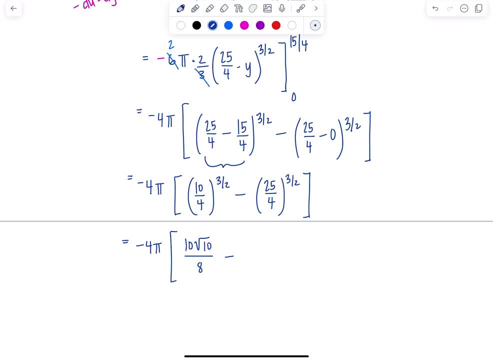 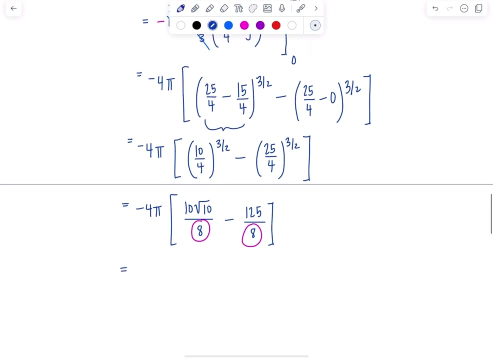 Minus square root of 25 is 5.. Cubed is 125 over 8 again, And then I can factor out the 8. And in fact I'm going to switch the order of subtraction and make everything positive. So I'm going to have positive 4 pi over. 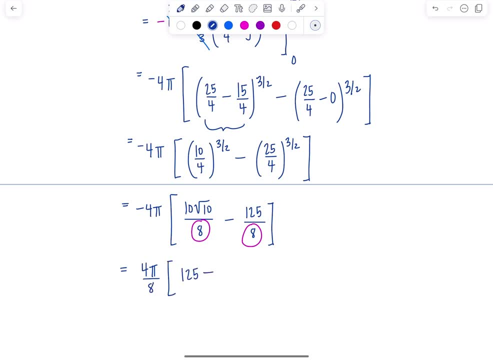 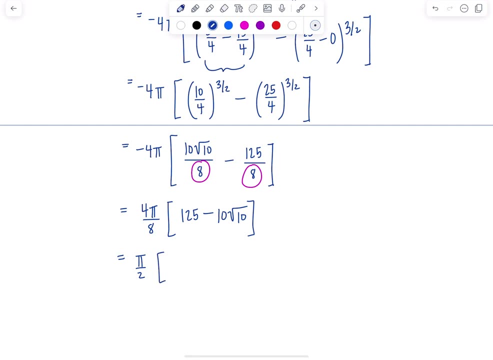 8. And then write it as 125 minus 10, rad 10,, you see, And then we just have pi over 2 times 1, 25 minus 10 rad 10.. You can leave it like that. That looks plenty fine to me. 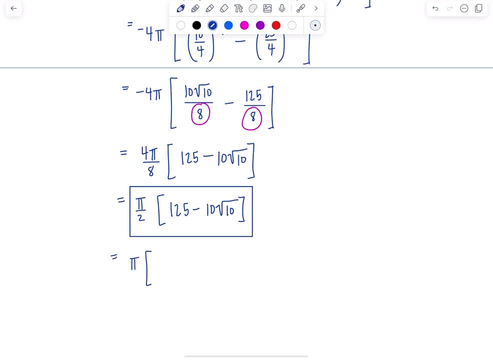 If you're inclined and you just only want to leave the pi out, then you have 125 over 2 minus 5 rad 10.. I don't think that looks a whole lot better. I don't know. They both look about the same to me. Which do you prefer, Option 1 or 2??